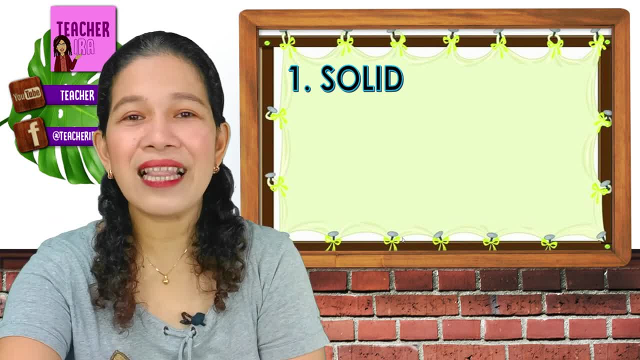 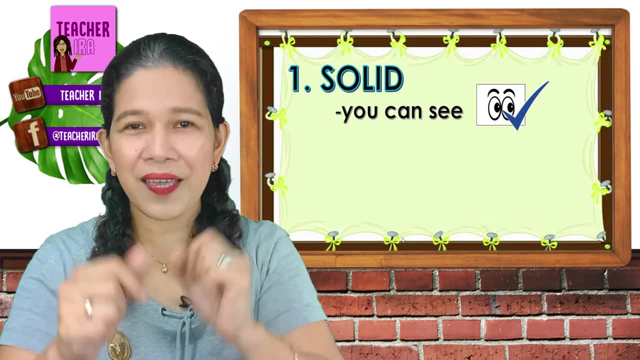 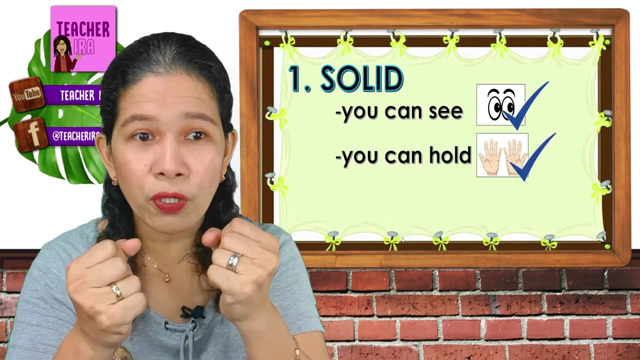 What are the characteristics of matter? What are the characteristics of solid things? Let's take a look at them one by one. First, solids are the things that you can see. Can you say that? You say you can see with your eyes. What else You can hold? Okay, anything that you can see and you can hold. 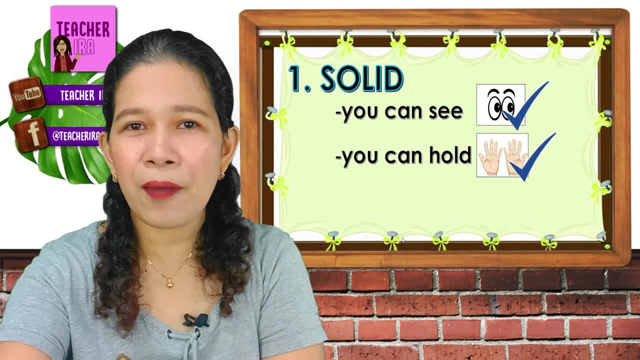 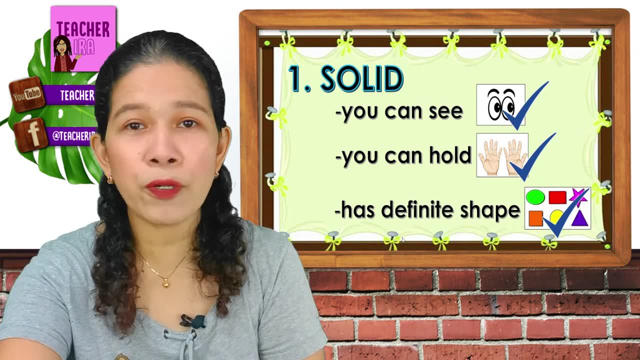 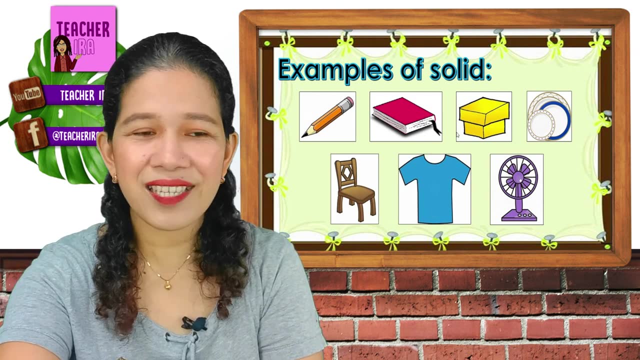 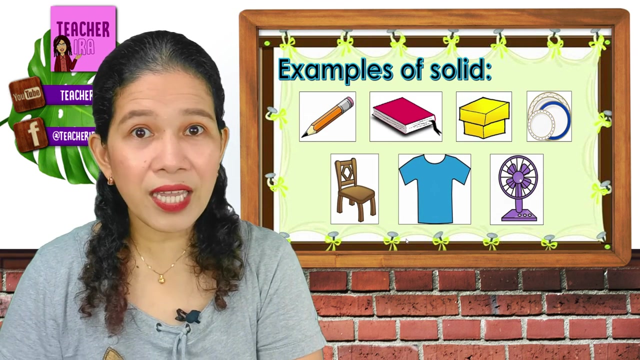 are called solids. Later I will give you some examples And one more. Solids have definite shape. Now let's take a look at the different examples Of solid. I have here: pencil, book, box, plate, chair, shirt, fan. These are all examples of solid. 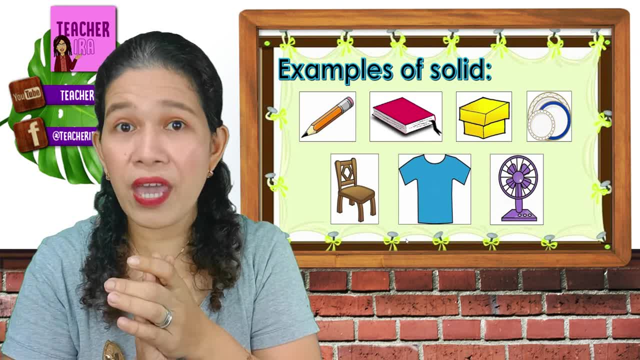 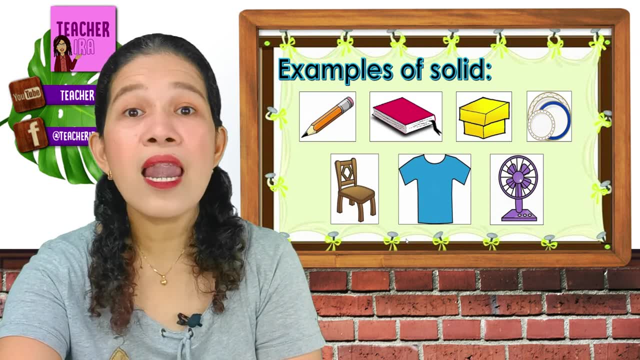 We can see them, We can hold them with our hands and they have definite shape. Let's call them solid. Now let's go to the second state of matter, which is liquid. You say a liquid. What are the characteristics of liquid? What are the characteristics of liquid? 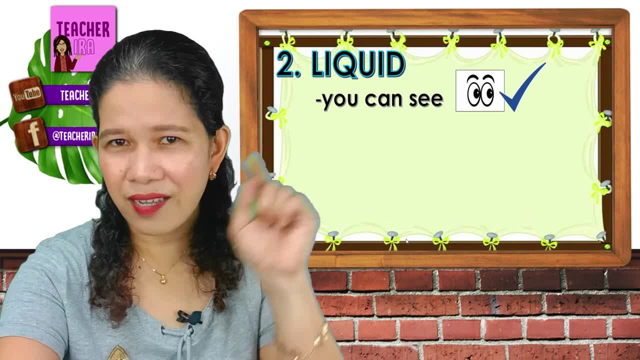 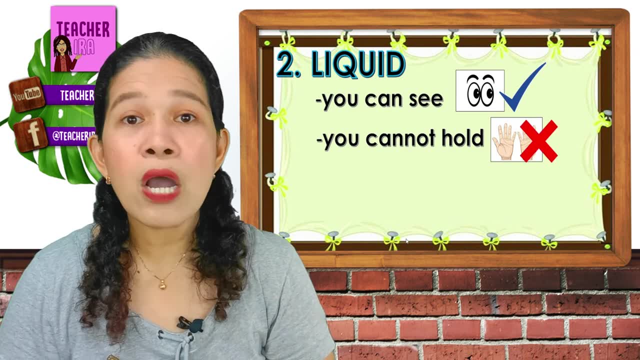 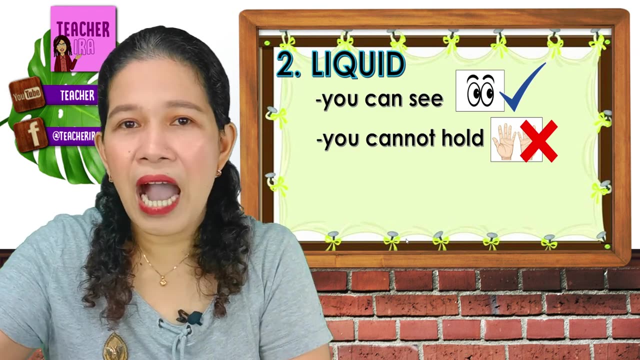 Number one. you can see. Check What else. Let's see if we can hold it. No, no, no, The liquid things. you may be able to touch it, but you cannot put it in your hands. Let's try. for example, I have here a bowl with water. 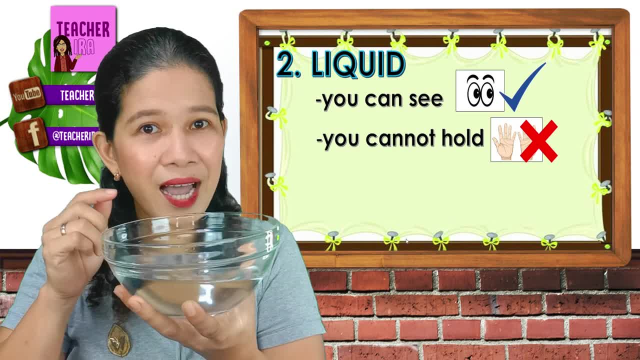 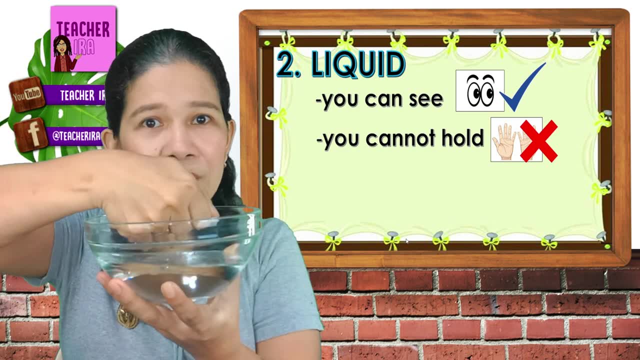 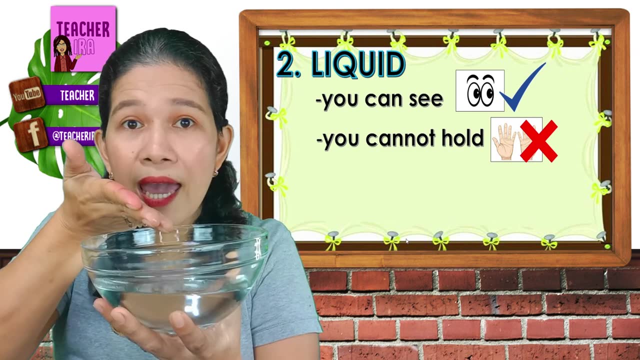 Water is one of the examples of liquid. Now I will try to get water. See, I can touch it. but let me try to get water And catch it No more, Because this is liquid And one of its characteristics is: you cannot hold it or you cannot put it here in your hands. 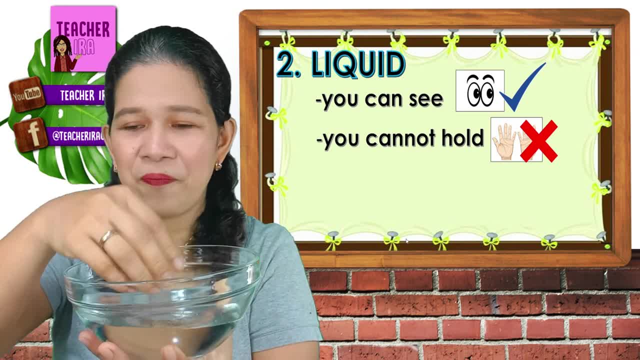 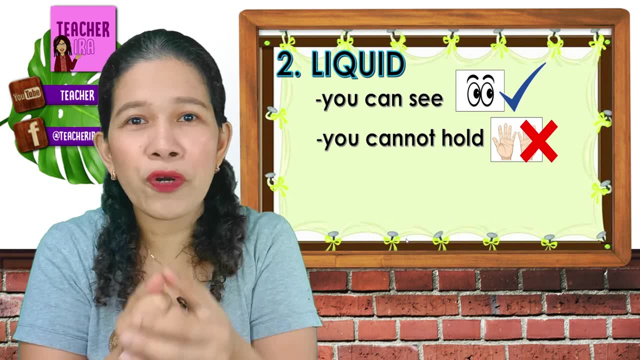 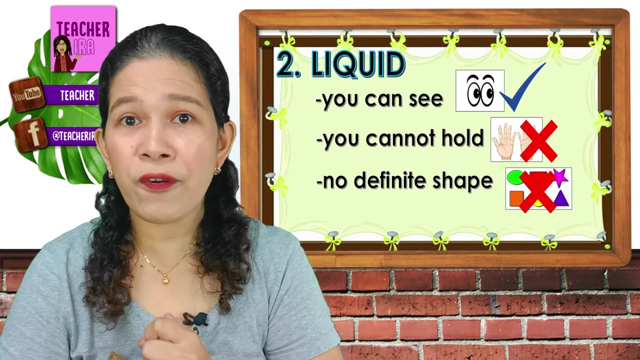 Look at that, Unlike the solid things, Hey, what else? So we said: we can see it, yes, but we cannot hold it or we cannot put it in our hands. Next, It has no definite shape. No definite shape, of course, because it follows the shape of its container. 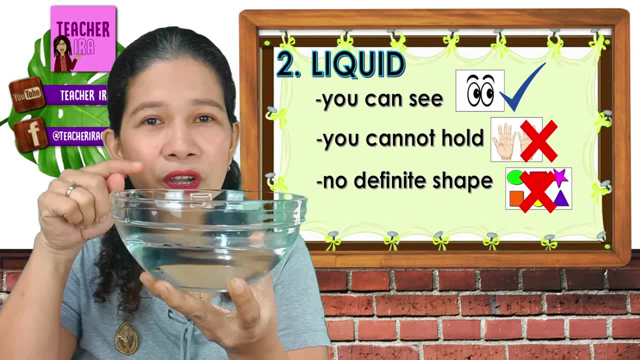 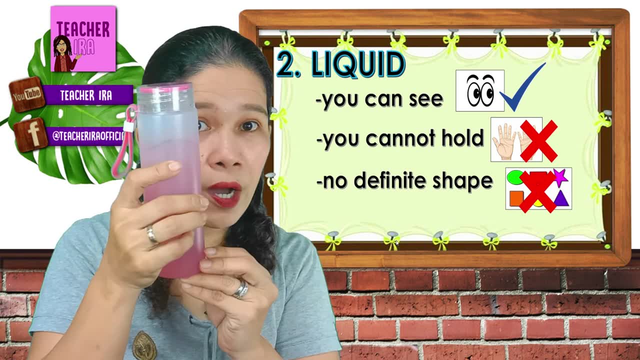 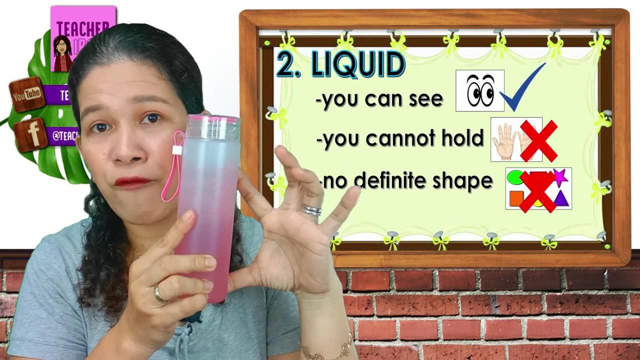 Remember this bowl that I've shown you a while ago. Look at the water inside, So it follows the shape of the bowl. I have another one here. I have this water bottle. Look at the shape of the water inside. now. It followed the shape of the bottle where I've placed it. 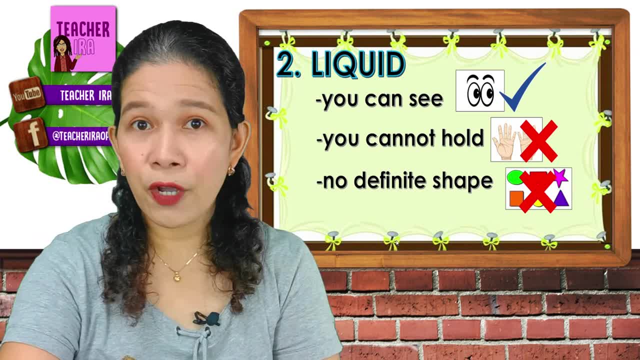 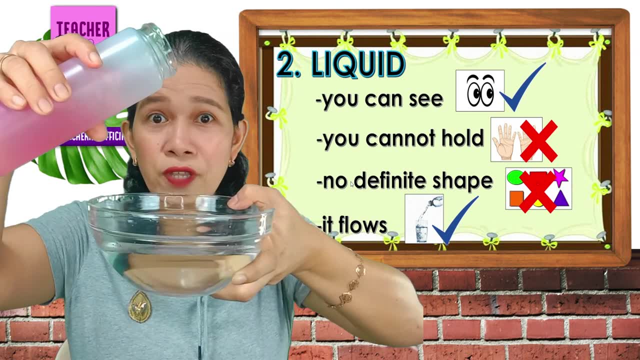 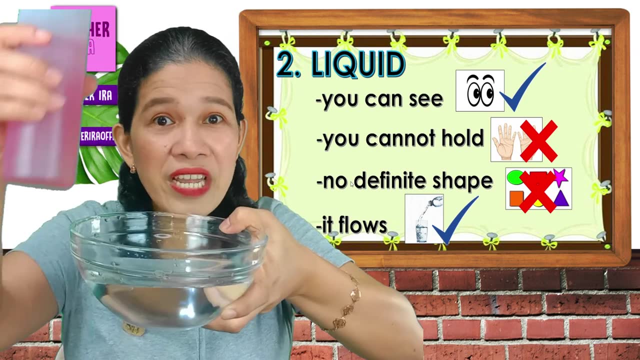 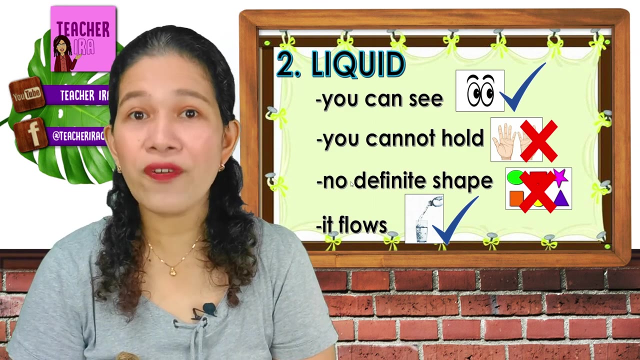 See that? One more thing: Liquids Flow. Let's take a look at this one. This has water inside and let's see if this will flow. See that The water inside spilled and it flows, because that's one of the characteristics of liquid. 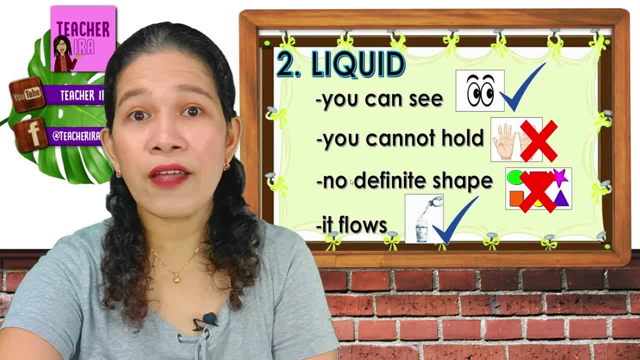 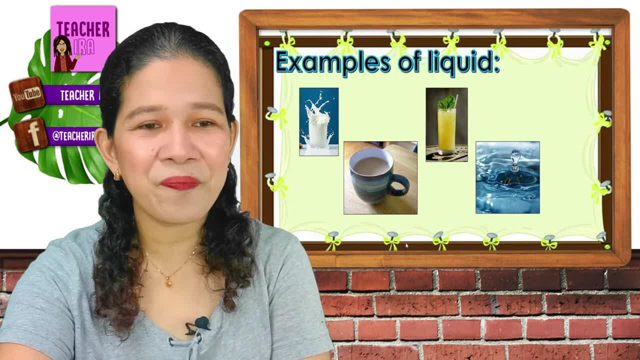 I have here more examples of things that are liquid. I have here fresh milk, coffee. It was mixed already in a cup. I have a juice there and water. These things flow. We already had the two, the solid and the liquid. 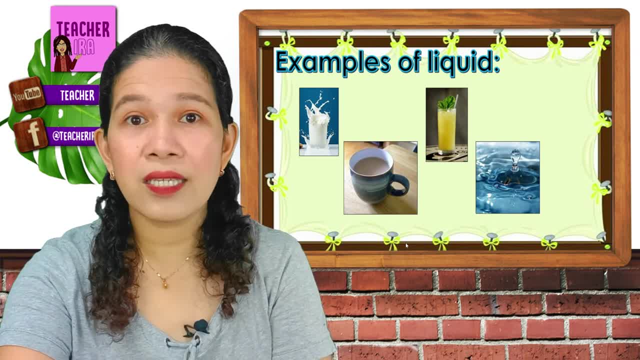 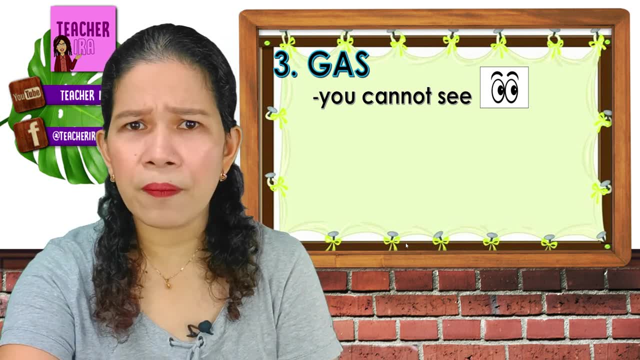 Now let us take a look at the third one. This is gas. You say gas, You cannot see. With a gas, you cannot see them. Next, You cannot hold, You cannot catch them or put them in your hands. Next, 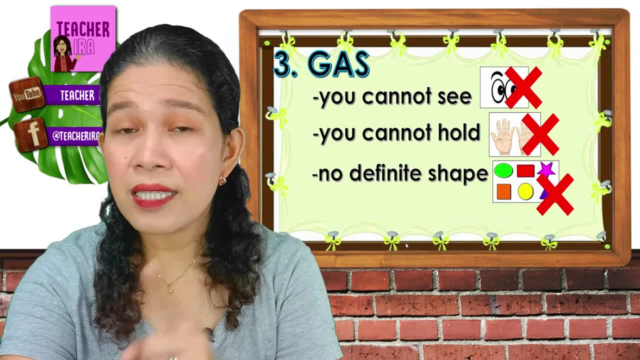 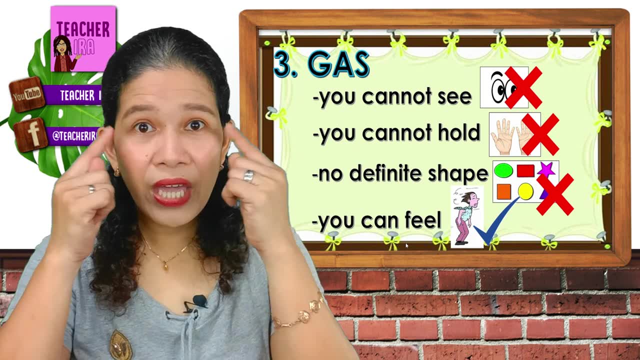 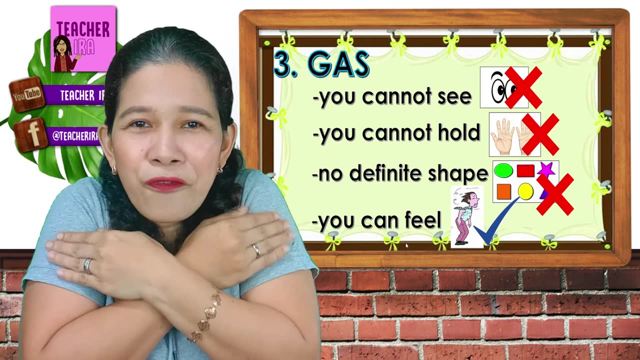 No definite shape Because the same with liquid, It follows the shape of its container. And you can feel, You say you can see, You cannot hold No definite shape, But you can feel. Now I want you to put your hands together like this: 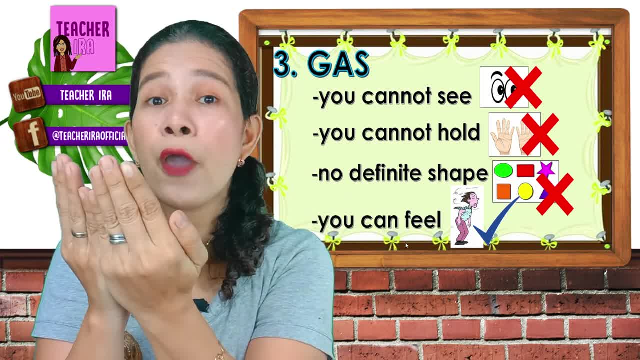 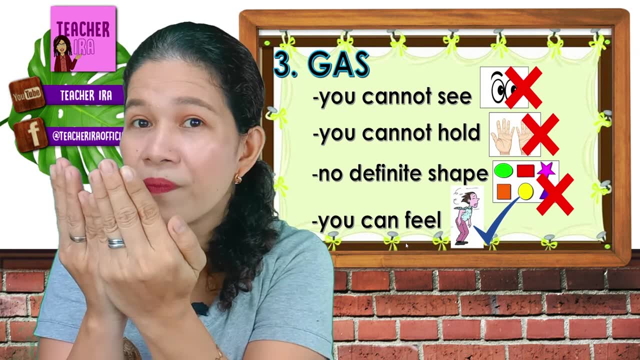 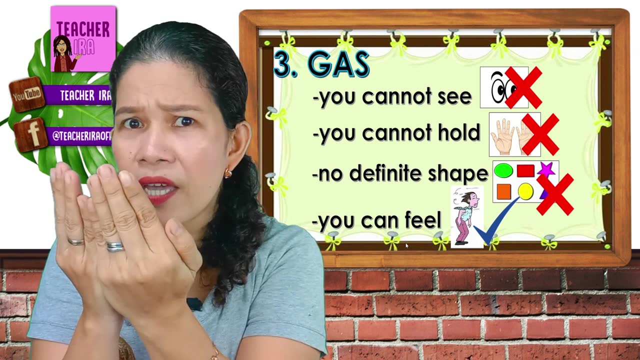 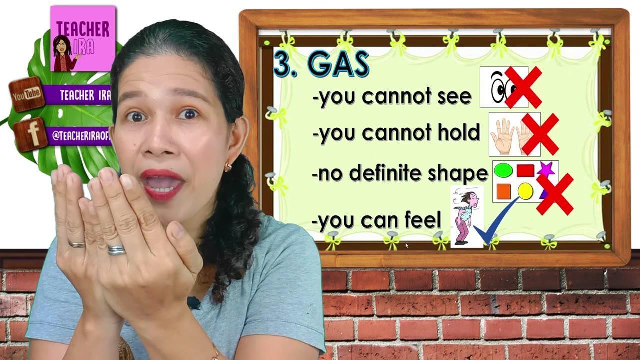 Now with your hands like this: I want you to blow hard on your hand. Go One more time, One more time. Now, let me ask you: Did you see the air? No, Now, try to catch the air now. 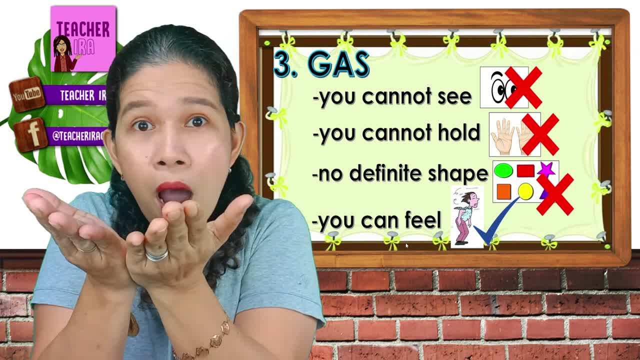 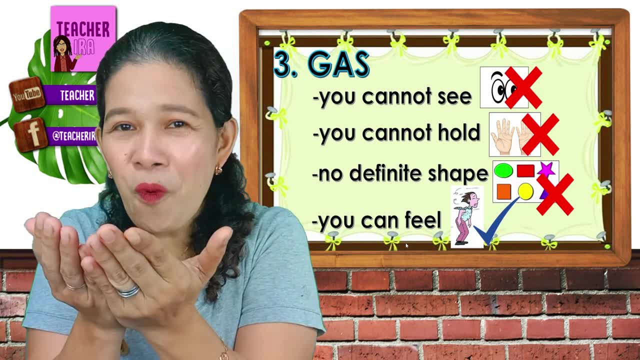 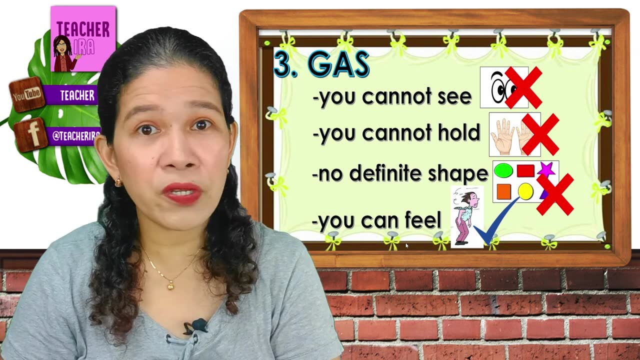 Close, Close, Close. Where is it now? There is nothing in my hands Because you cannot hold it. Next One more time You blow. Can you feel it Great? Because that's one of the characteristics of the gas. 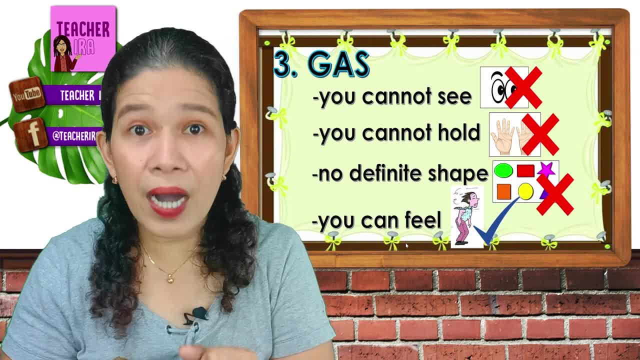 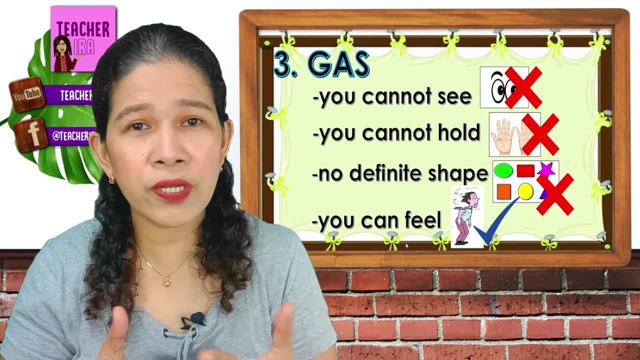 You may not be able to see it, You may not be able to hold it, But you can feel it. Imagine you are in front of an electric fan or an air-conditioned unit. Could you feel the air? Yes, But you cannot see it. 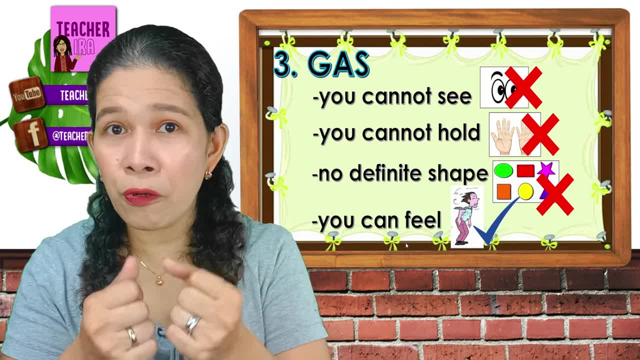 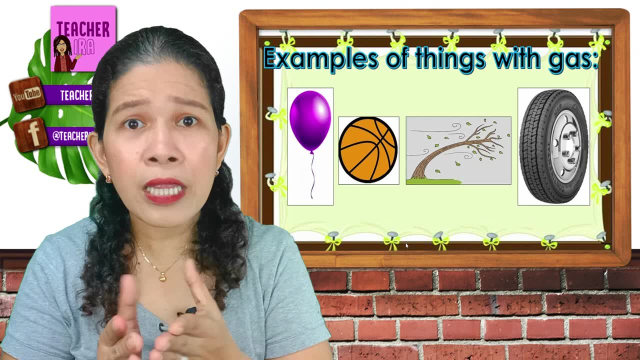 Definitely you cannot see it, Definitely you cannot hold it or put it in your hands. I have here examples of things With gas inside. They may be solid from the outside, But let us talk about the things that are inside. Let us have this balloon. 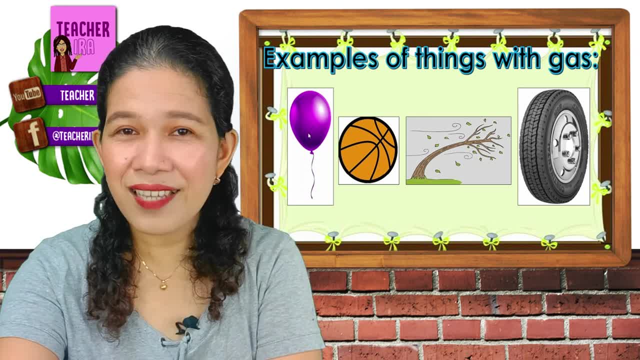 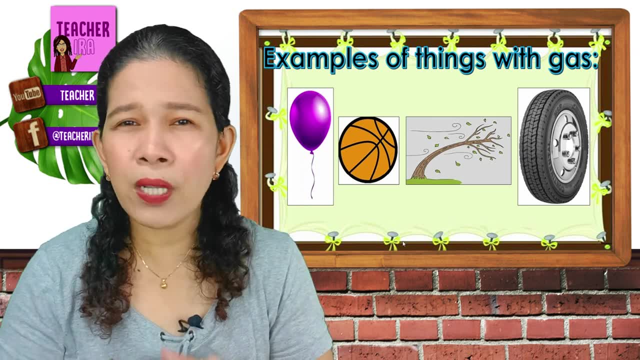 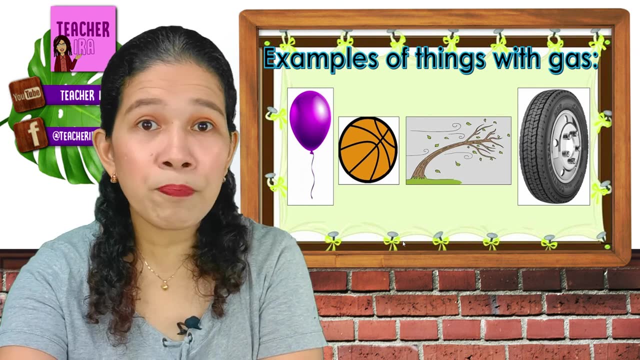 This balloon has gas inside. That's air, Children. it changes shape. Have you seen balloon with heart shape? Or balloon that is oblong in shape Because gas follows the shape of its container? Look at this ball Here. it has gas or air inside. 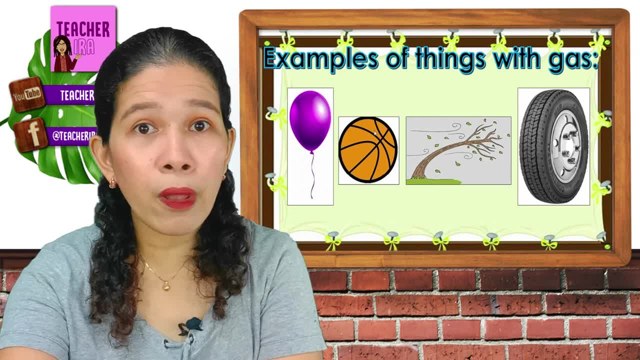 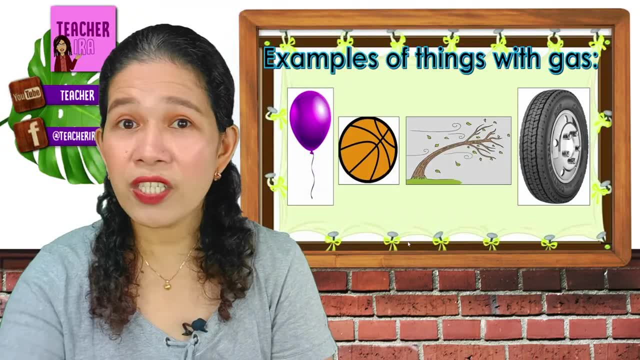 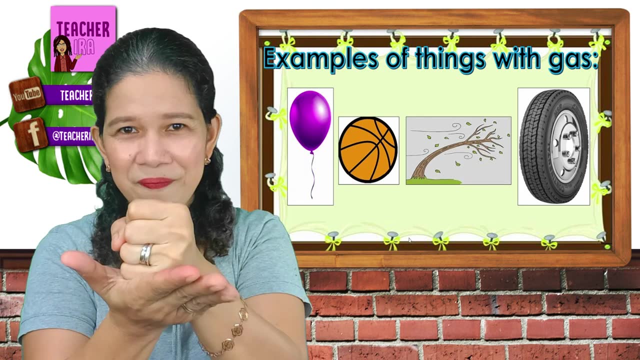 And the wind that is blowing is also a kind of gas. The tire has gas inside. So, children, today we have learned about the three states of matter. Let's name them again. Say solid, Now let's have liquid and then gas. 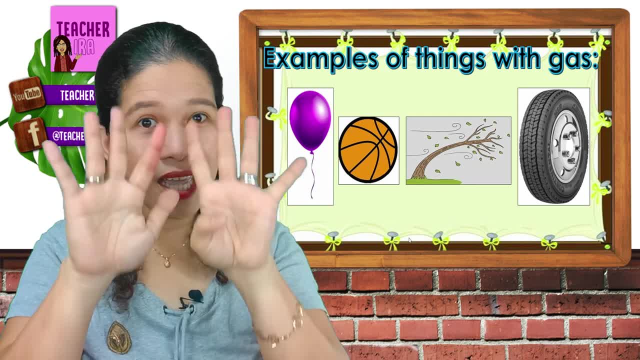 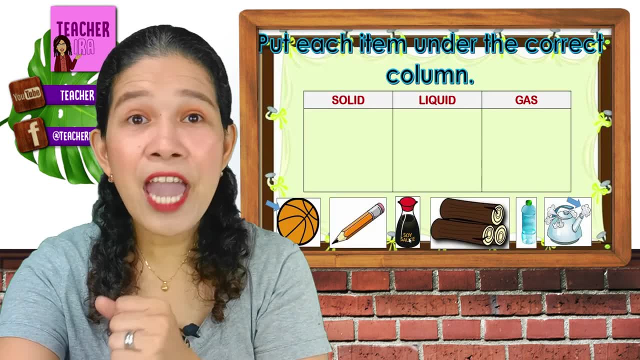 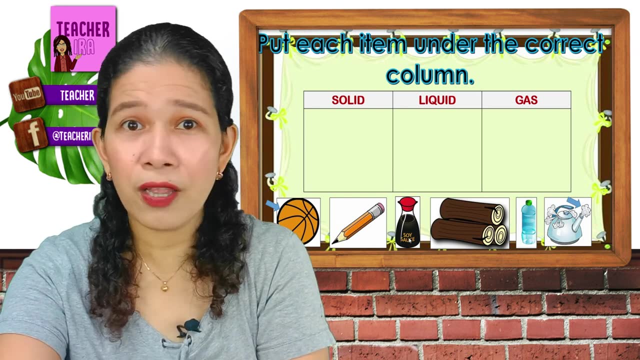 One more time: Solid liquid gas. Now teacher Ira would like to know You can get this one. I have here examples of things. I want you to put them in the right box. Is it solid, liquid or gas? 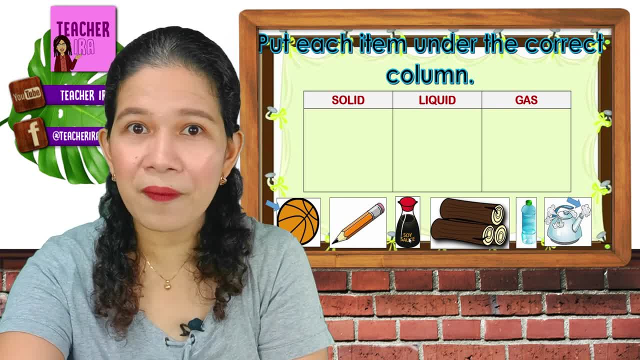 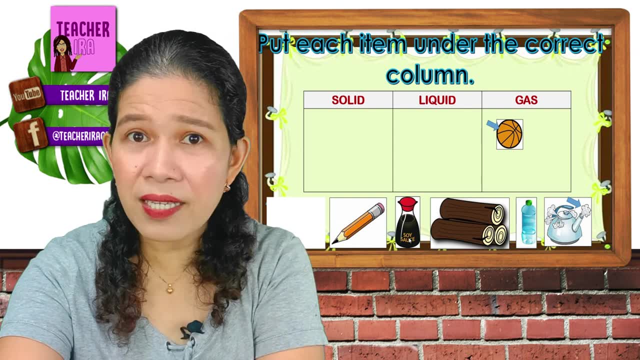 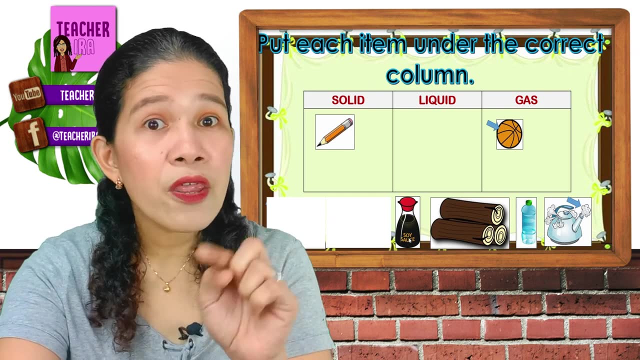 Let us begin with the ball. What is inside the ball? You are correct, It's gas. How about this pencil? Yes, it's solid. How about the soy sauce that is inside the bottle? So let's talk about the soy sauce inside. 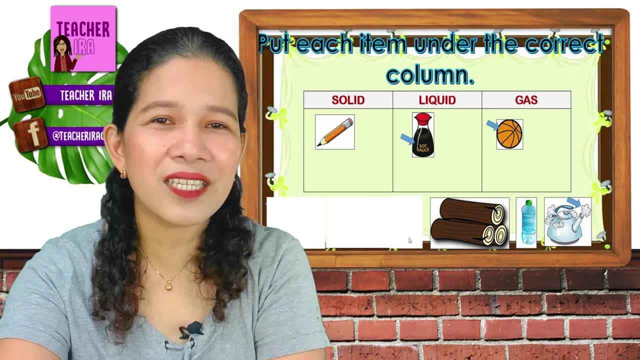 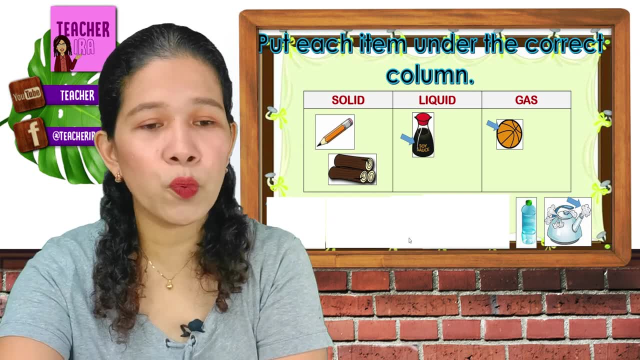 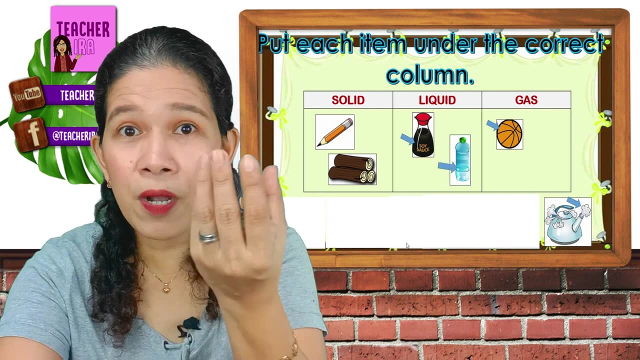 Yes, it's liquid. How about the lump? Yes, that is definitely solid. And how about the water inside the water bottle? It's liquid. And last, the steam coming from the boiling water. What do you think? Can you see it? 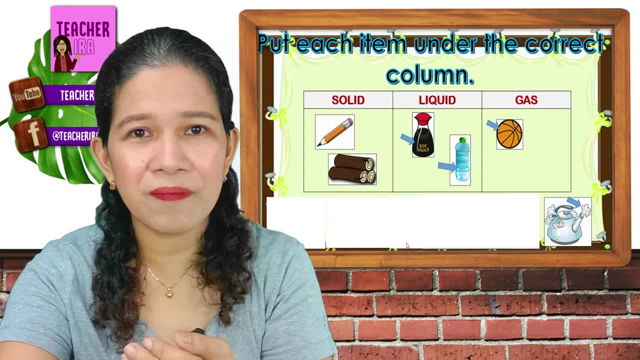 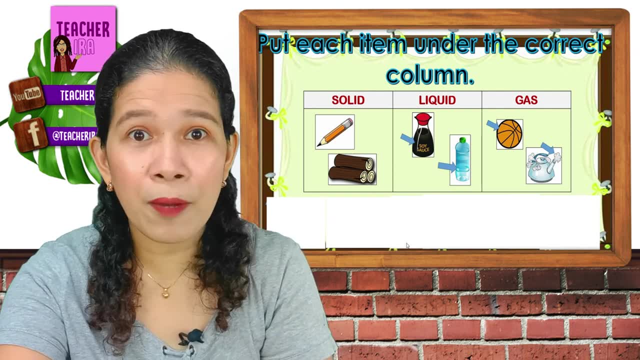 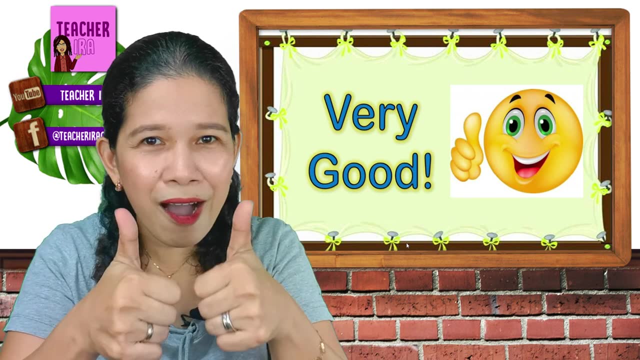 Can you feel it? Can you touch it? Let's see. Yes, that's definitely gas. So, kids, here are some examples of things that are solid, liquid and gas. You did a very good job. Thank you so much for listening today, kids.